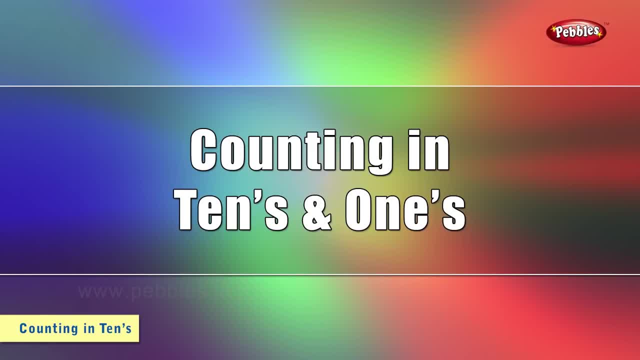 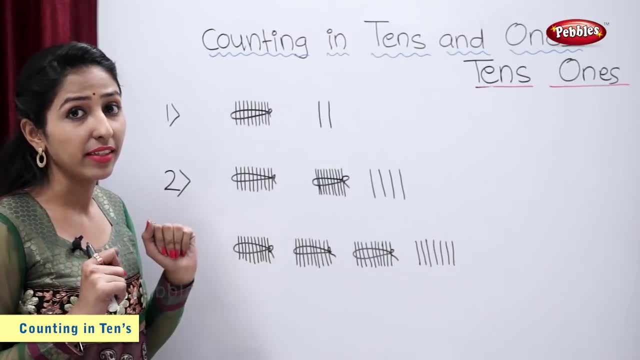 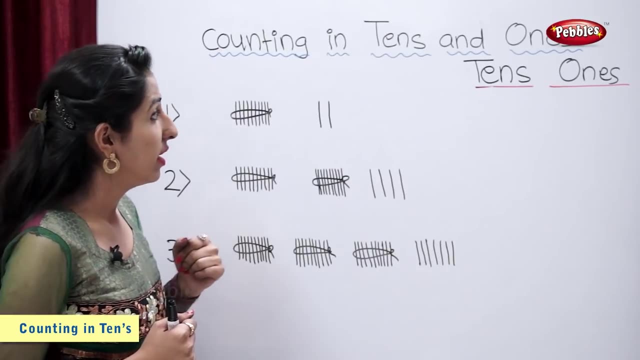 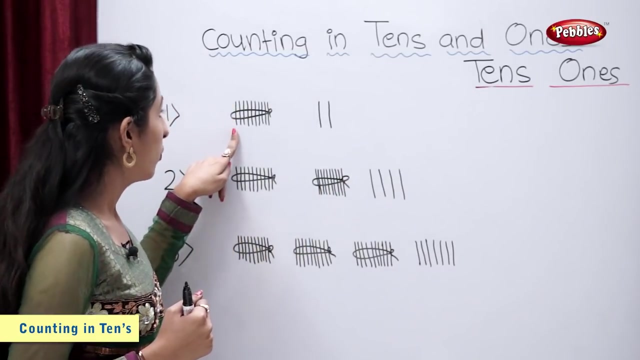 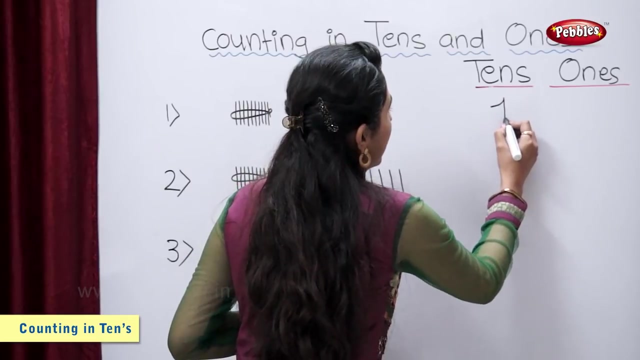 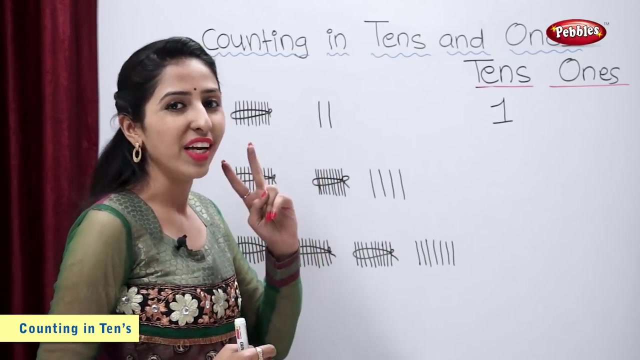 Counting in 10s and 1s. Here I have 1 bundle of 10 sticks and 2 loose sticks. So tell me, students, there are how many 10s and how many 1s. We have 1 bundle of 10 sticks, So we have 1 10s. We have 2 loose sticks, So we have 2 1s. 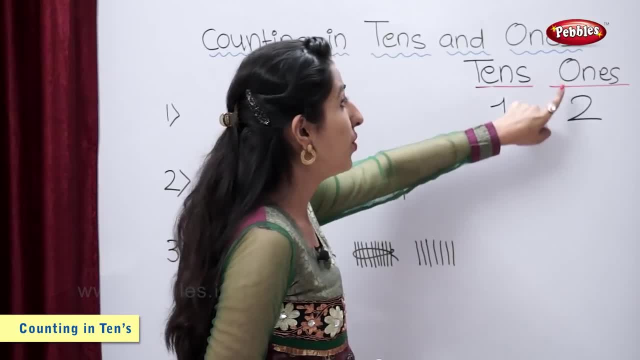 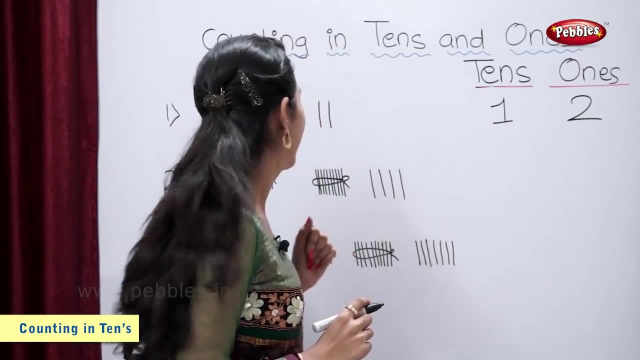 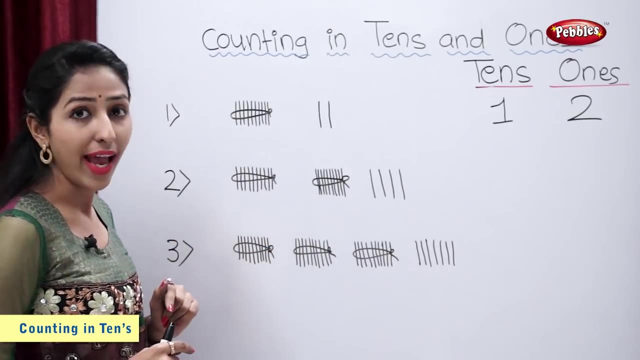 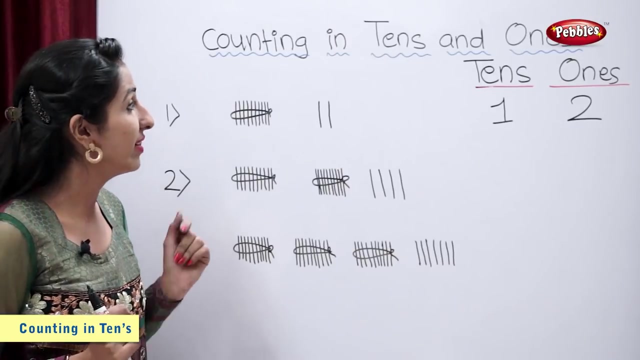 1 10s, 2 1s, So the number is 12.. Here there are 2 bundles of 10 sticks and 4 loose sticks. So tell me, students, there are how many 10s? 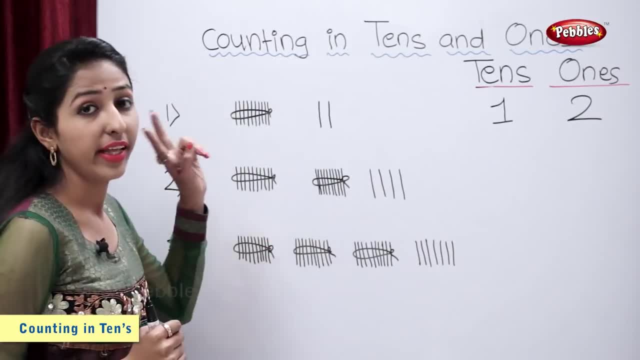 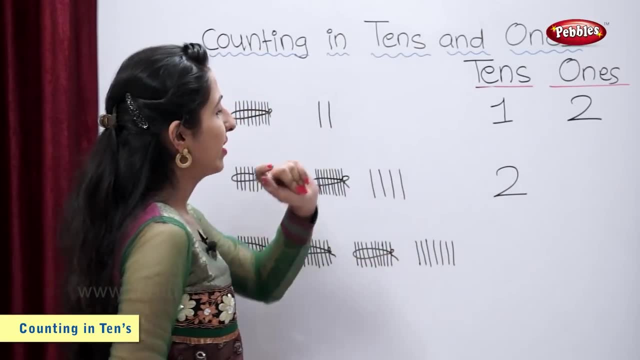 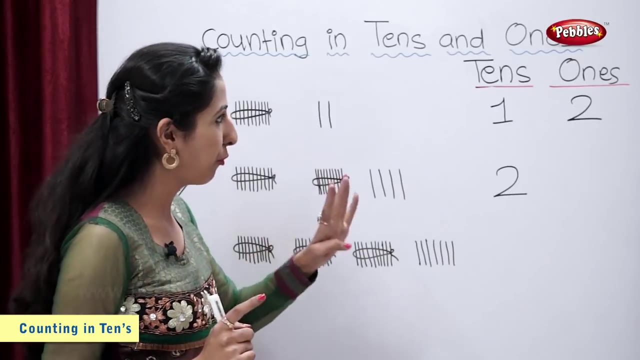 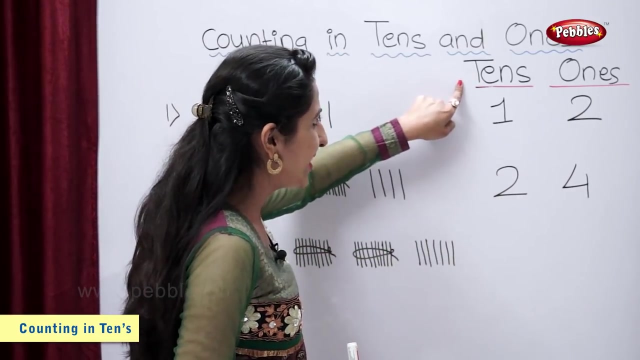 1 and 2.. There are 2 bundles, So 2 10s. 1, 2, 3, 4.. 4 loose sticks, So 4 1s. 2 10s, 4 1s, So the number is. 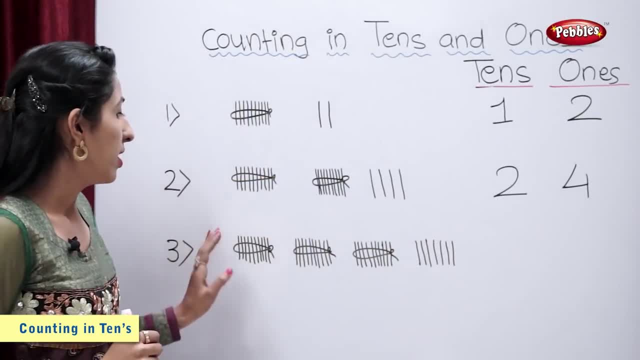 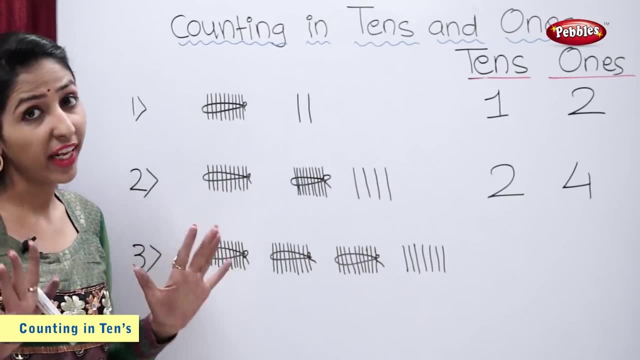 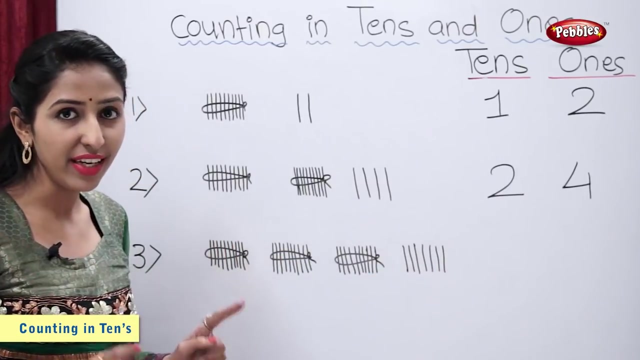 24. Here I have 1,, 2,, 3., 3. 3 bundles of 10 sticks and 1,, 2,, 3,, 4,, 5,, 6,, 7. 7 loose sticks. So we have 3- 10s. 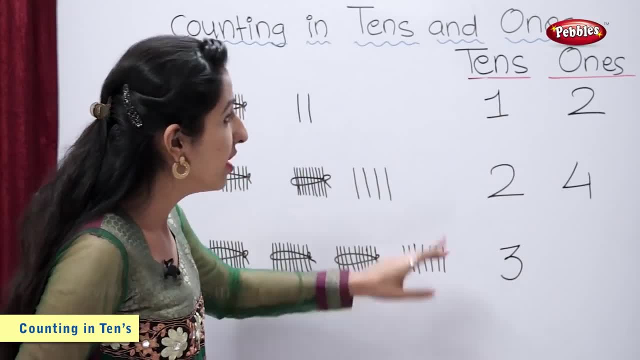 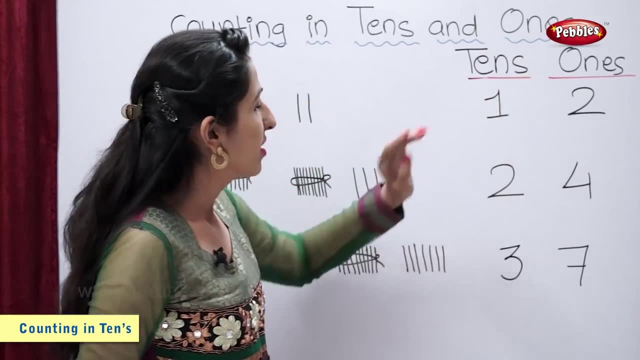 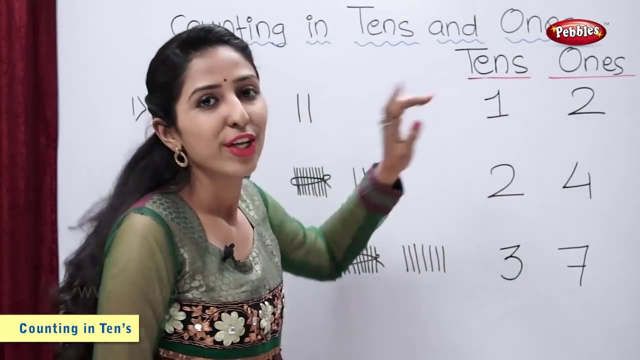 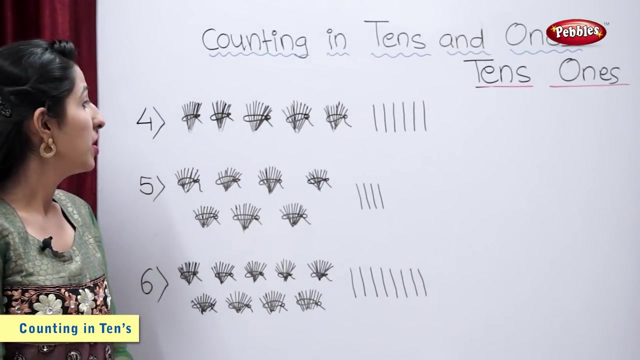 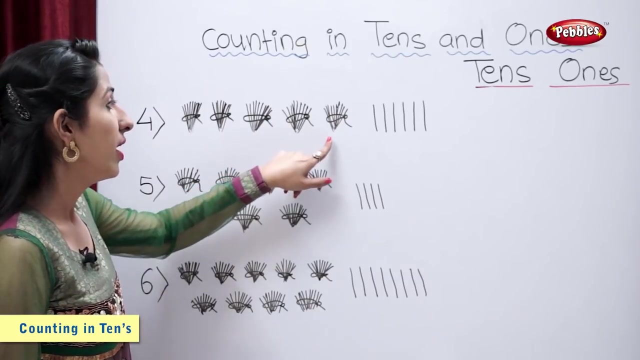 3 10s and 7 1s, 7 1s, 3 10s, 7 1s. So the number is 37.. Now we have 1,, 2,, 3,, 4 and 5.. 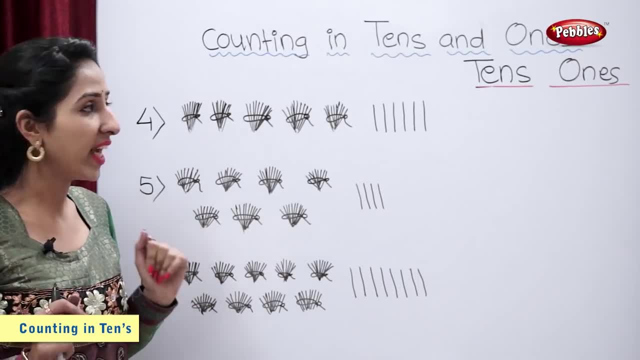 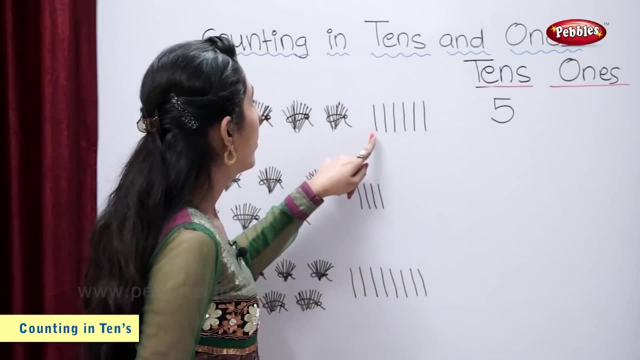 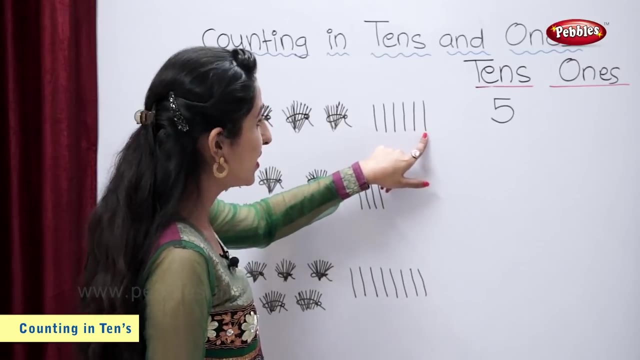 5 bundles of 10 sticks, So we have 5 10s. 1,, 2,, 3,, 4,, 5 and 6. 6 loose sticks, So we have 6 1s. 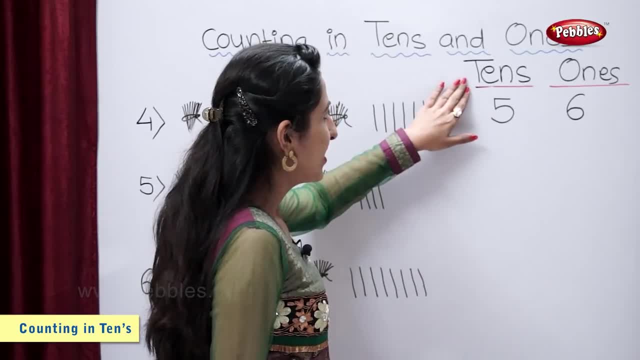 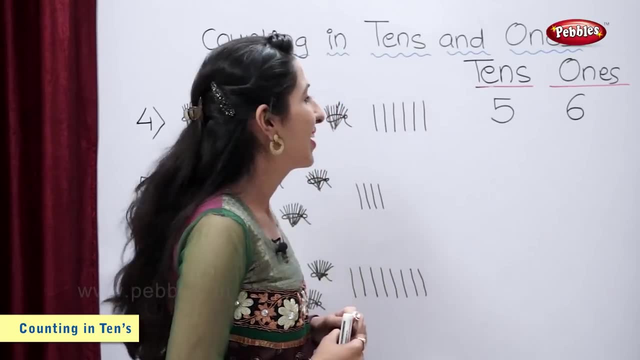 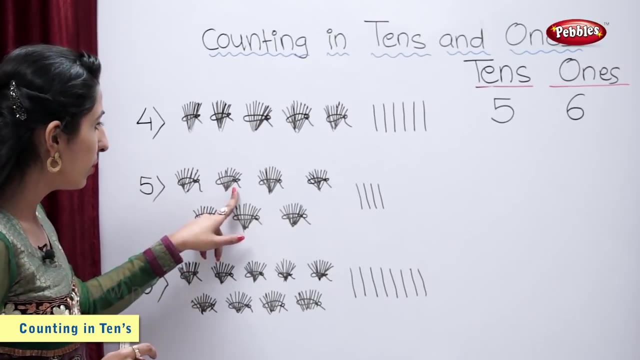 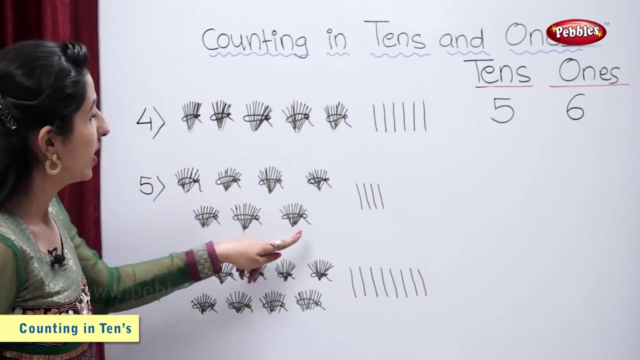 5, 10s, 6, 1s, So the number is 56.. Here there are 1,, 2, 3,, 4,, 5, 6 and 7.. 7 bundles of 10 sticks. 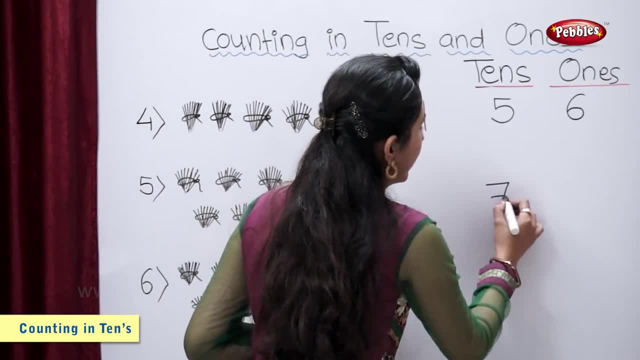 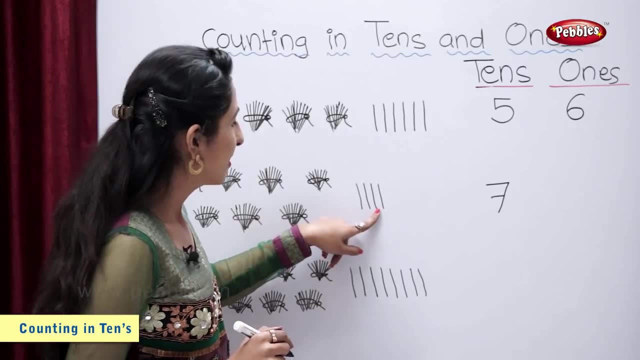 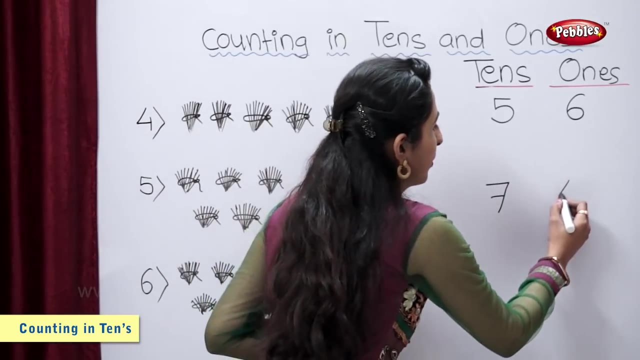 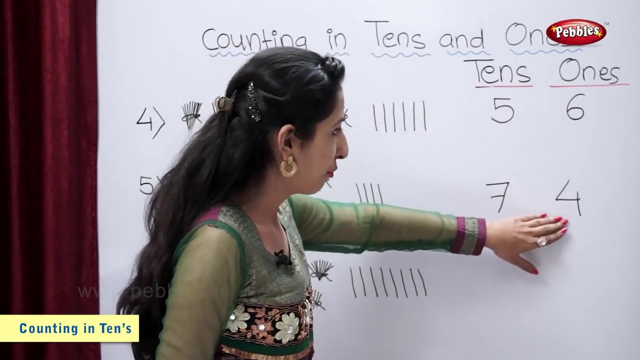 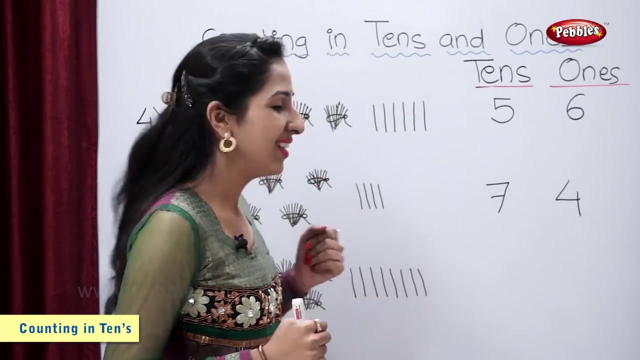 So we have 7 10s and 1,, 2,, 3 and 4.. 4 loose sticks, So we have 4 1s. 7 10s, 4 1s, So we get number 74.. 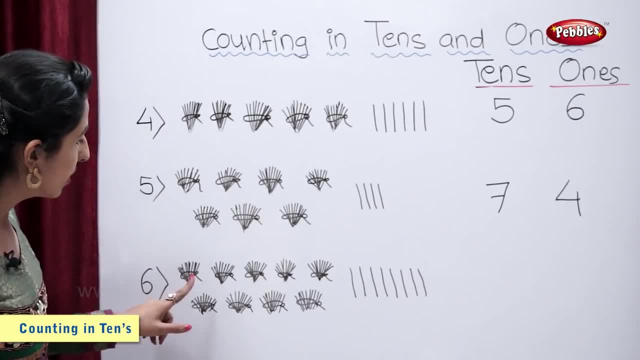 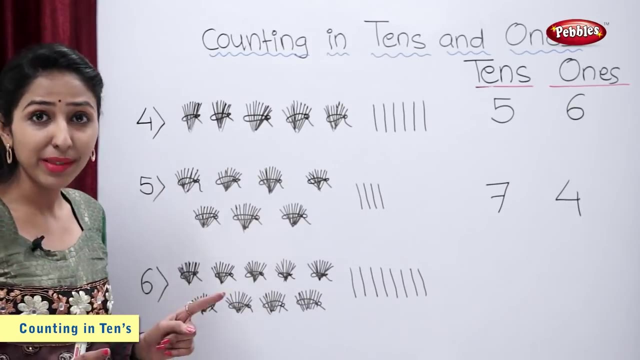 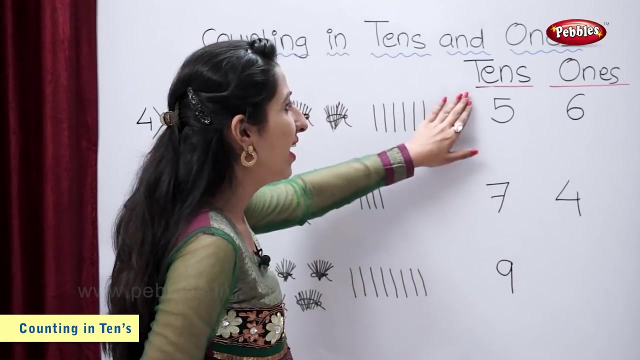 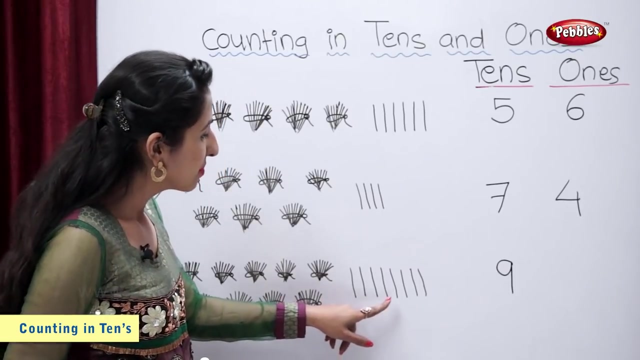 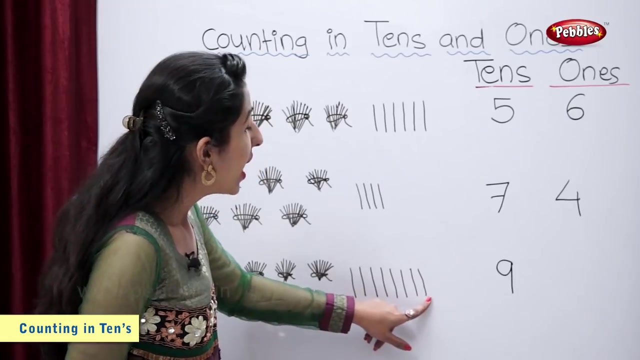 Here there are 1,, 2,, 3,, 4,, 5,, 6,, 7,, 8 and 9.. 9 bundles of 10 sticks. So we have 9 10s and 1,, 2,, 3,, 4,, 5,, 6,, 7 and 8.. 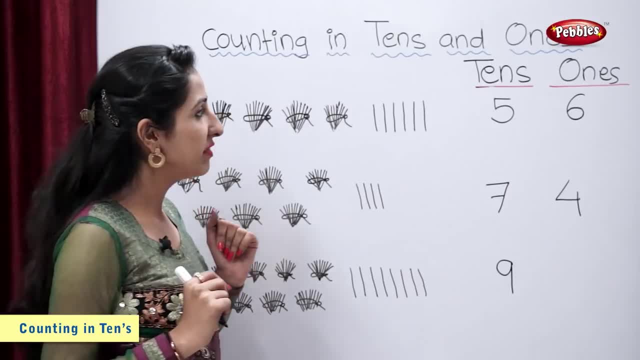 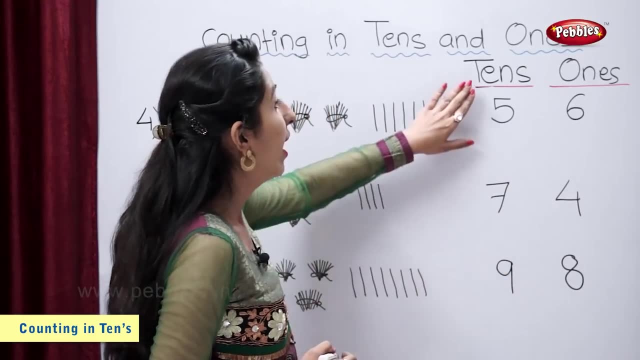 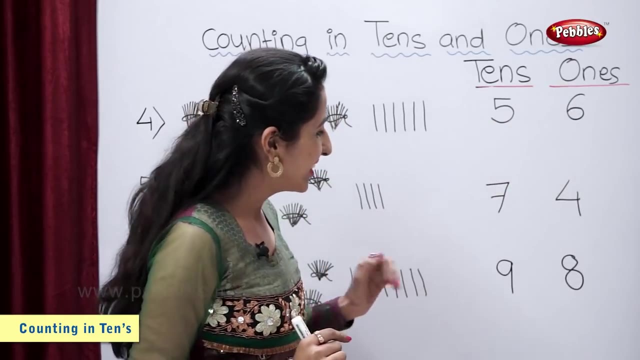 8 loose sticks, So we have 8 1s, 9 10s, 8 1s, So the number is 98..